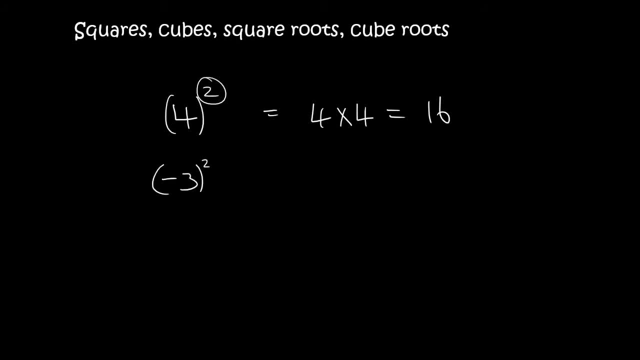 If I say minus 3 with a 2 there, it means minus 3 squared, and that means minus 3 times minus 3.. Now a negative and a negative is a positive, and so that is 9.. So negative 7 squared means minus 3.. 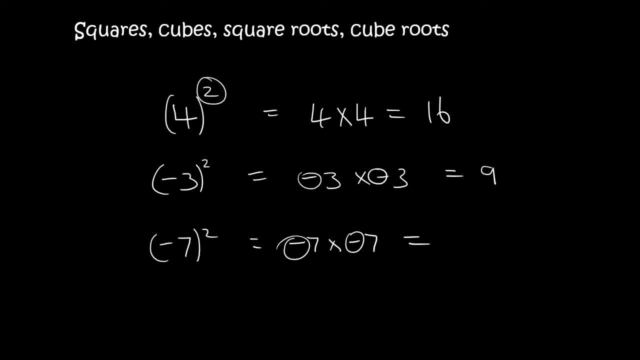 So if I say minus 7 times minus 7, a negative and a negative is a positive, If I have minus 1 squared, it means minus 1 times minus 1, which is 1.. So now, if I have minus 2 to the power of 3, it means minus 2 times minus 2 times minus 2.. 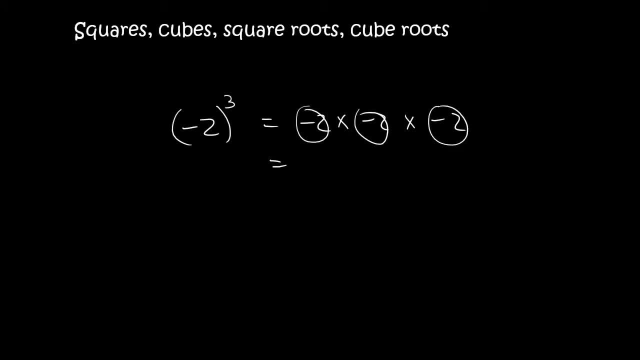 And we know that 2 times 2 is 4, times 2 is 8.. We then count the negatives 1,, 2,, 3. And so that will be a negative, Because it's an odd number of negatives. 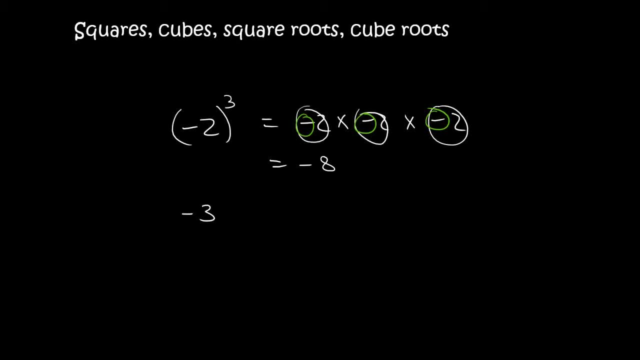 So it's negative 8. If you have minus 3 to the power of 3, that means minus 3 times minus 3 times minus 3.. And so 3 times 3 is 9, times 3 is 27.. 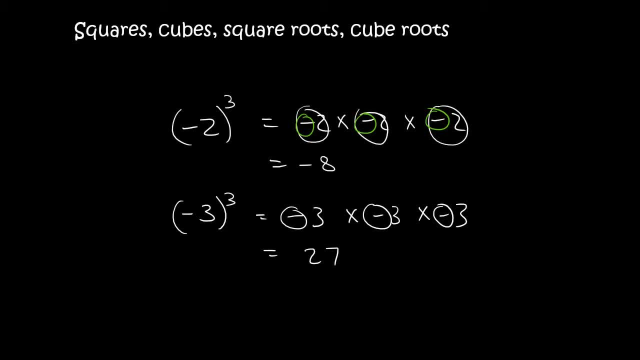 And then there's 1,, 2, 3 negatives. 3 negatives makes a negative. Now, if I give you something like this, we call this a square root, And so what this is saying is: what times? what gives you 4?? 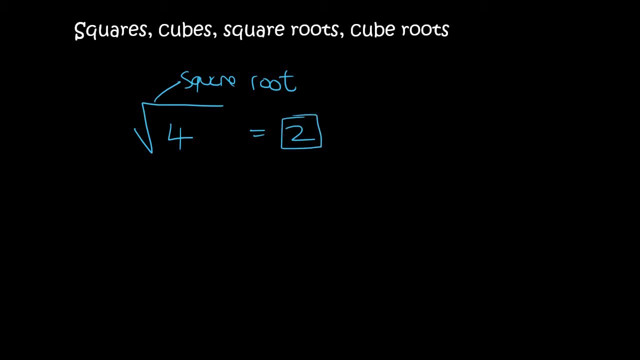 Well, 2 times 2 gives me 4.. So that is the answer 2.. This is saying: what times? what gives you 9?? Well, 3 times 3 gives you 9.. So the answer is 3.. 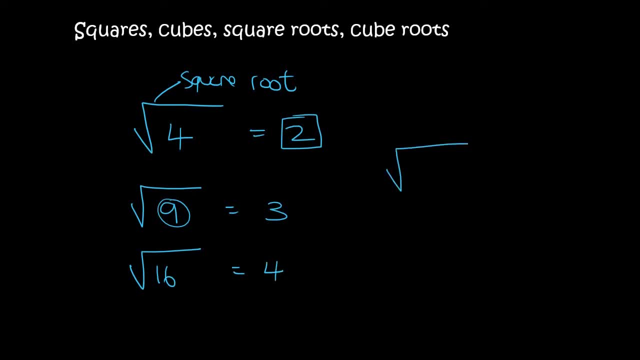 What times? what gives you 16? 4.. And let me quickly prove it to you. For this one over here, we know that 2 times 2 is 4.. For this one over here, we have: 3 times 3 equals 9.. 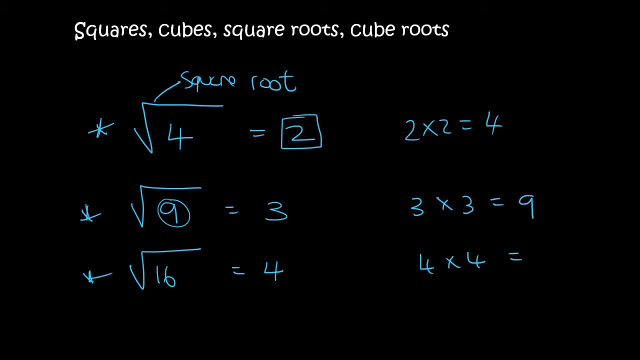 And then for this one. here we know that 4 times 4, is equal to 16.. Now, what about this one? Some people want to say that this is minus 2.. Okay, well, is minus 2 times minus 2 equal to minus 4?? 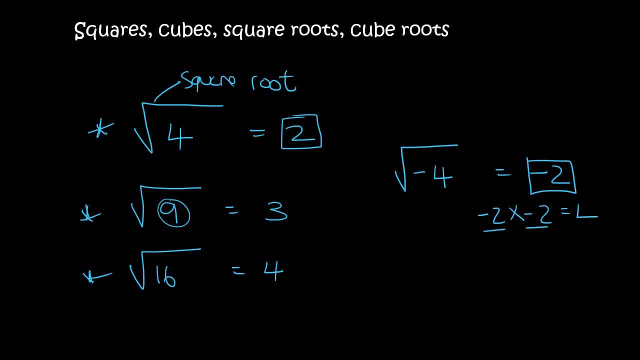 No, it's not, because minus 2 times minus 2 is positive 4. And so it is impossible to have a negative inside a square root, And so we give this, we call it- no real solution. So you can't have a negative inside a square. 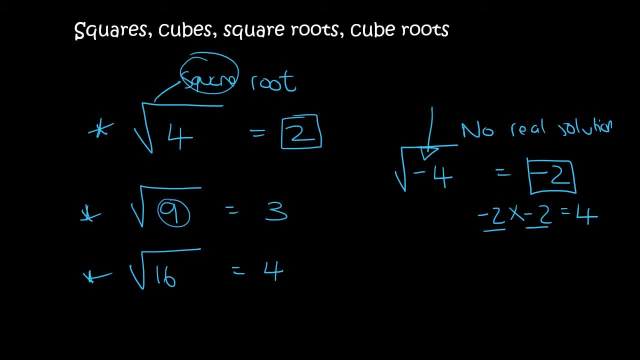 So you can't have a negative inside a square root. A cube root is different. Cube roots have a 3 at the top And they will have numbers such as 8.. So what this means is what number times by itself, 3 times, gives you 8?. 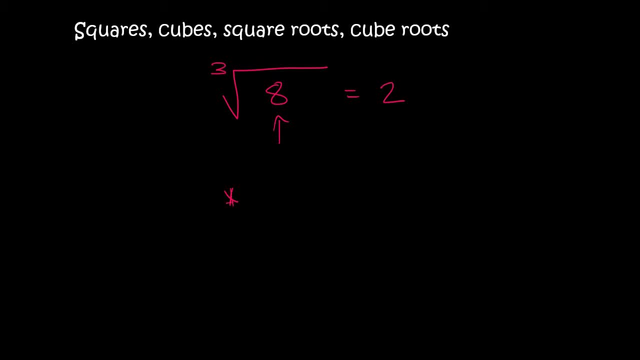 Well, that is 2.. Don't believe me: 2 times 2 times 2.. 2 times 2 is 4.. 4 times 2 is 8. 27.. So, what times, what times? what We do? 27.. 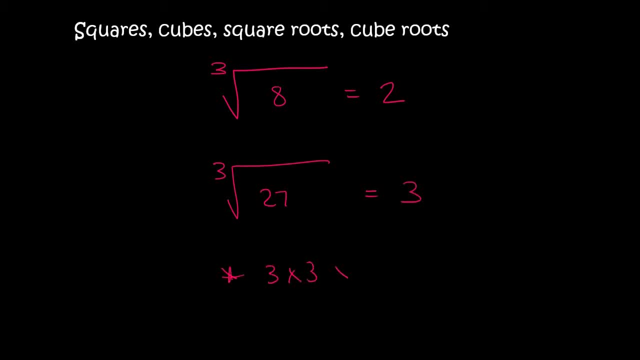 Well, that's the number 3.. Let's make sure: 3 times 3 times 3.. 3 times 3 is 9.. Times by 3 is 27. Minus 8.. Ah, so can you have a negative with these ones? 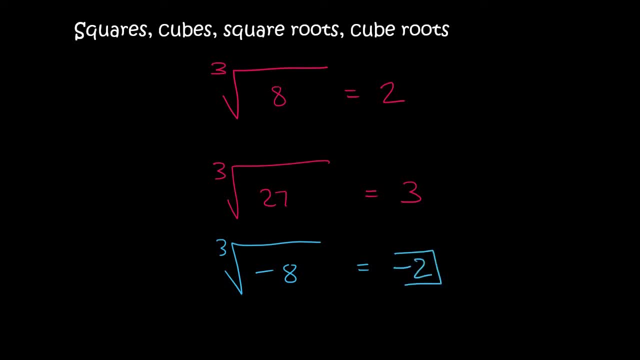 Well, let's see What if I told you that the answer was minus 2? Let's see: Minus 2 times minus, 2 times minus 2.. Well, 2 times 2 times 2 is 8.. 3 negatives makes a negative. 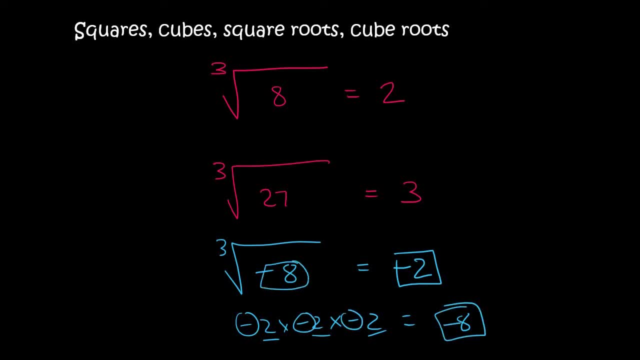 And so, yes, we can. So we can have a negative inside a cube root, but you can't have a negative inside a square root. See the difference: A square root looks like this and a cube root looks like that. It's got a 3.. 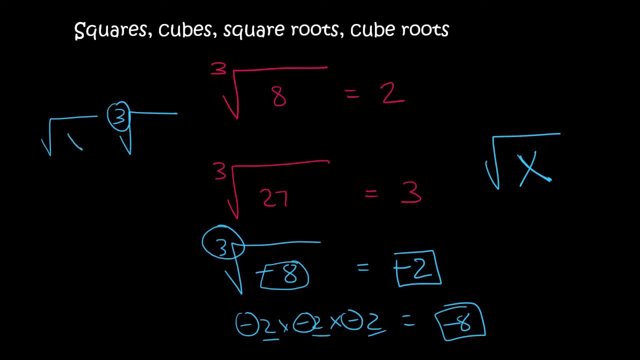 So you can't have a negative inside a square root, but you can have a negative inside a cube root. So here's a question. Let's call this number 1.. So we can do this part by itself. We can do this part by itself because there's a times. 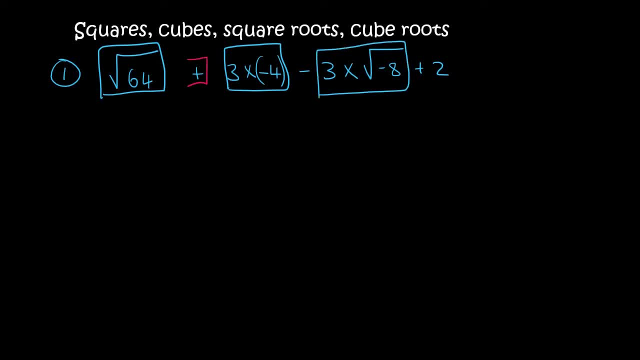 And then we can do this whole part by itself, And then we'll just leave the plus, this minus and this plus 2 for the end. So here we have the square root of 64.. So it means: what times? what gives you 64?? 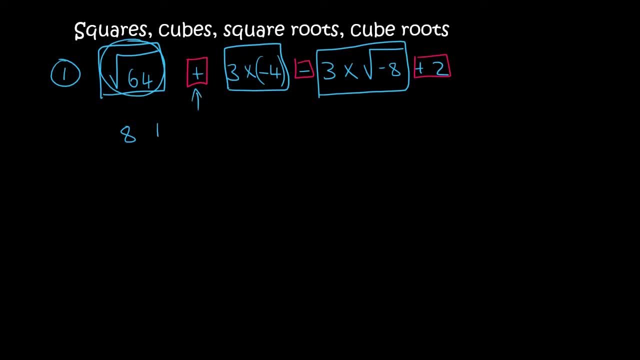 Well, that's 8. Then I'm just going to write down the plus. Then the answer inside this next block is 3 times 4. But there's one negative, so that's minus 12.. So I'll just put minus 12.. 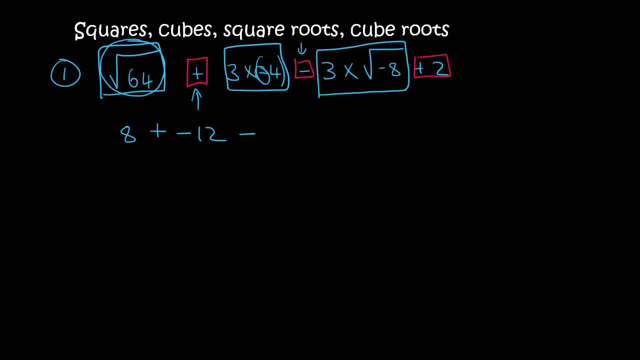 Then there's a negative, Then I've got this: Oh, there should be a cube over there, My bad Cube root of minus 8.. So what times? what times? what gives you minus 8? That's minus 2.. So inside this block, we've got 3 times minus 2, which is minus 6.. 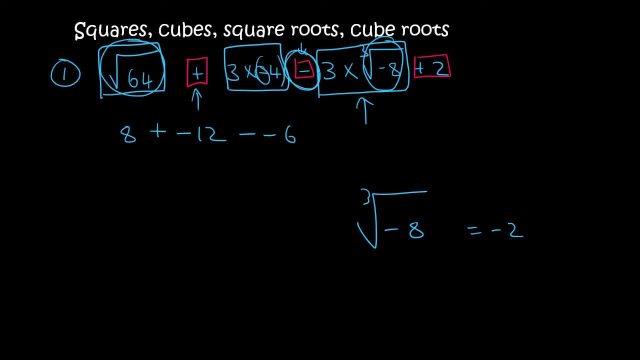 So I've already written this negative down, So I'm just going to put negative 6 next to it and then plus 2.. Now we can just simplify the positives. So a positive and a negative is a negative, A negative and a negative is a positive. 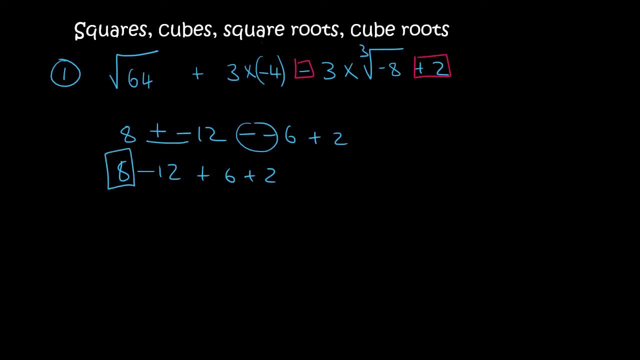 We now go from left to right. If you have 8 rand and you give away 12 rand, then you have minus 4 rand. If you have minus 4 rand, so you owe people 4 rand. and then someone kindly gives you 6 rand. well, now at least you have 2 rand. 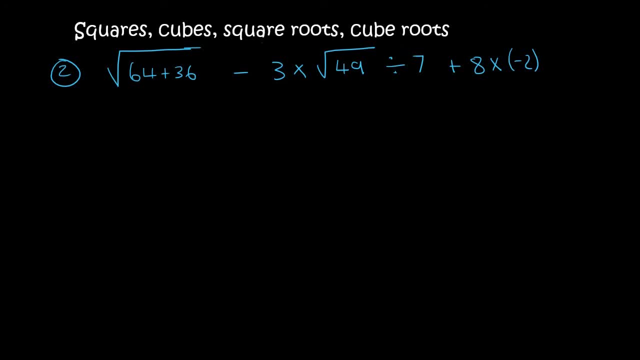 Then 2 plus 2 is 4.. Moving on to number 2. So we could break it up into this part, Then this part, And then this part. See, so it's usually the minuses and the pluses that get left alone. 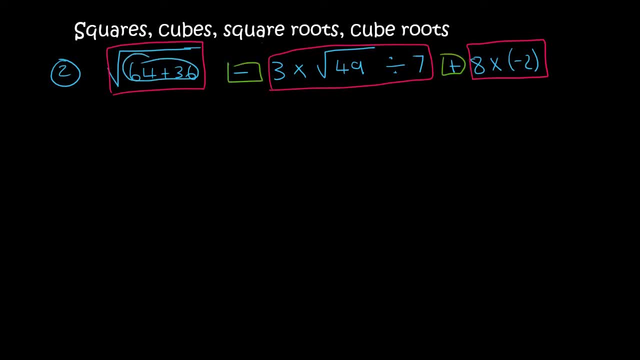 So we know that 64 plus 36 is 100. And the square root of 100, so let's look at that- is 10.. Why? Because 10 times 10 is 100. So I can just write this as a 10.. 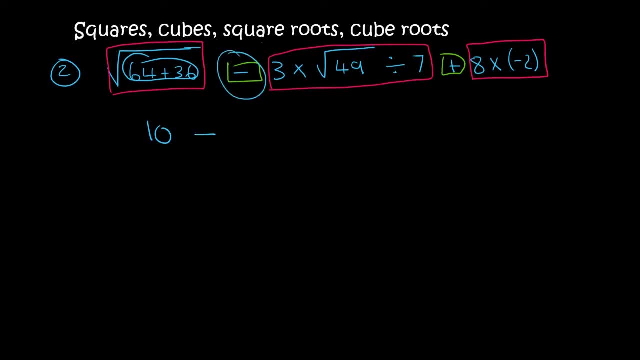 I can then write down this minus. Now I can do everything inside The second block. So that's 3 times square root 49 divided by 7.. That's 3 times now the square root of 49 is 7, because 7 times 7 is 49.. 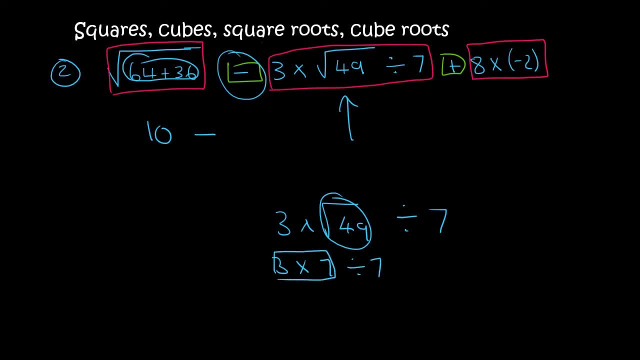 Now I move from left to right. 3 times 7 is 21.. 21 divided by 7 is 3.. So this entire block is 3.. And then there's a plus over here, And then 8 times 2 is 16, but there's a negative, so that's negative 16.. 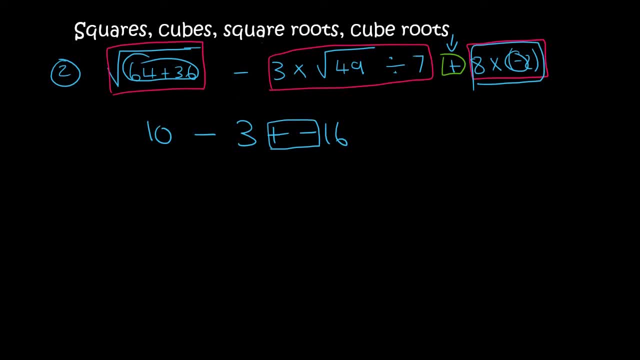 Notice. it's completely okay to write a plus and a minus next to each other, Because in the next line I can change that A plus and a minus is a minus. 10 minus 3 is 7.. Now if you have 7 rand and you give away 16 rand, that's minus 9..